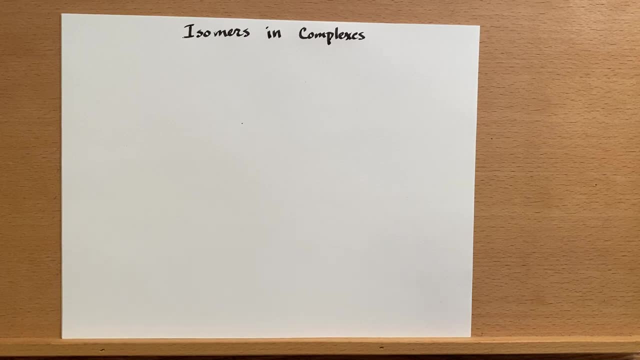 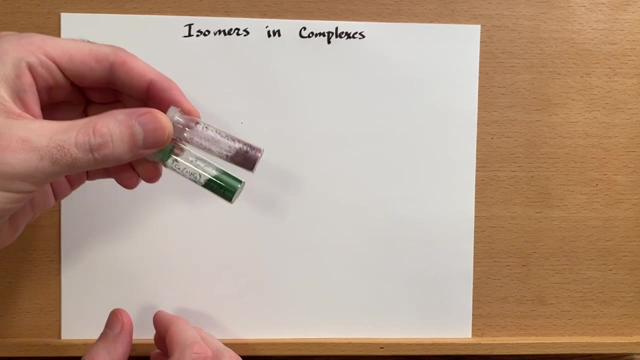 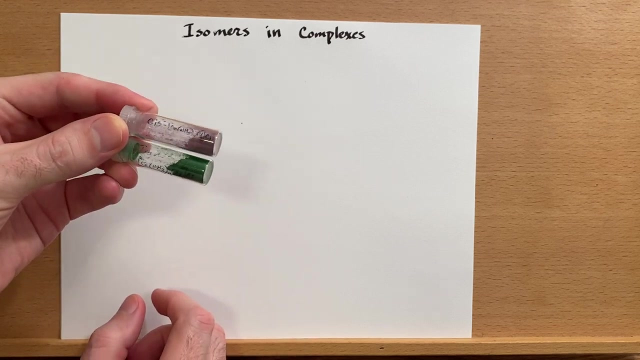 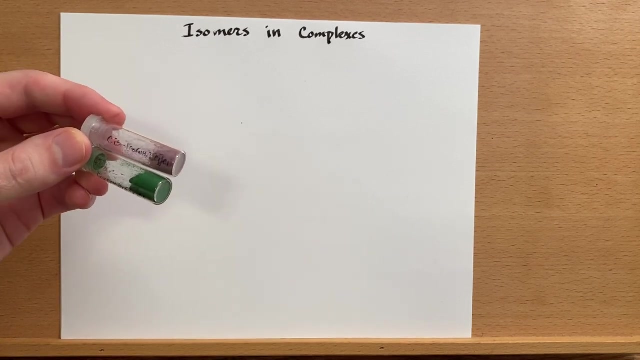 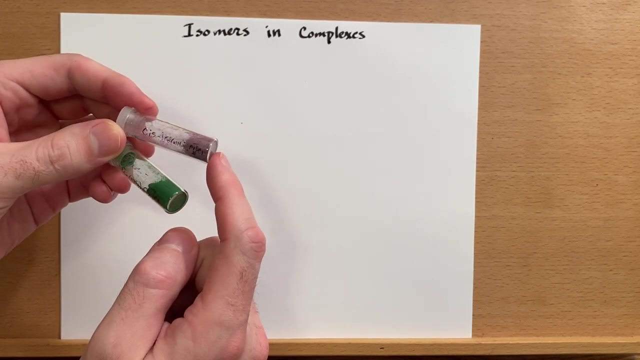 Let's talk about isomers in inorganic complexes. So, as an example here, I actually have two isomers and you'll see that one of them's purple and the other one's green, And these have the same chemical formula and it is tetra-amine-dichloro-cobalt-3-chloride, And the purple one is the cis configuration and the green one is the trans configuration. 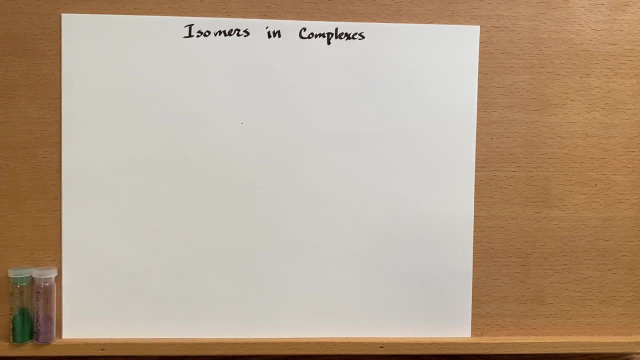 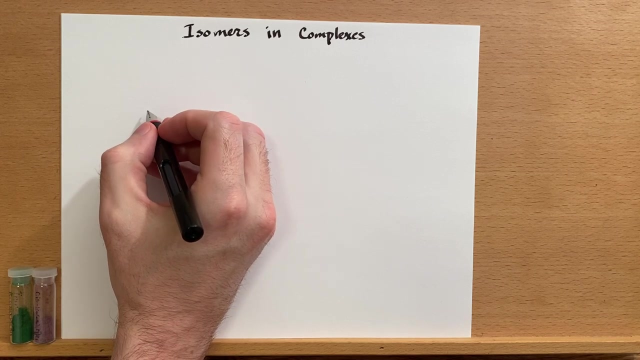 So let's draw out what those configurations look like and discuss a few. There are two other isomers that we can have when we're looking at inorganic complexes, So let's start off by drawing the cis configuration or the purple compound. 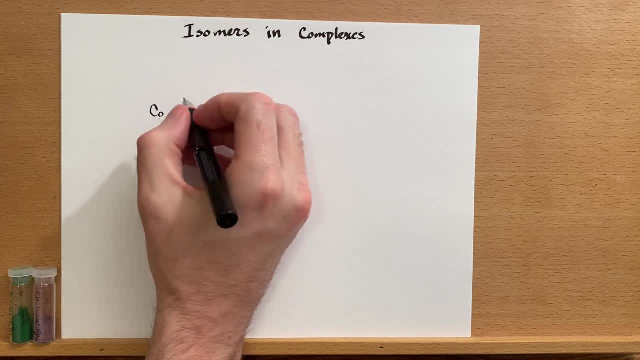 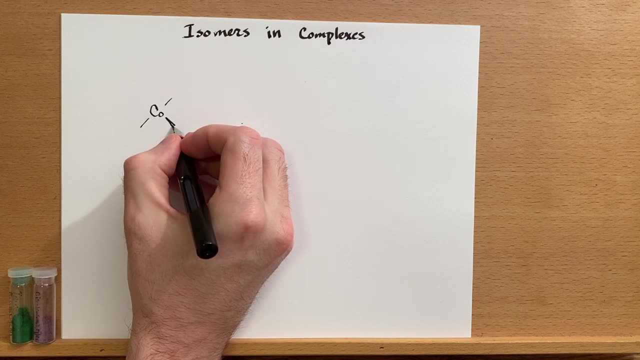 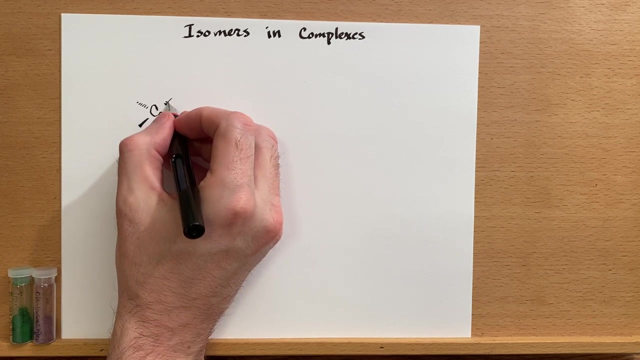 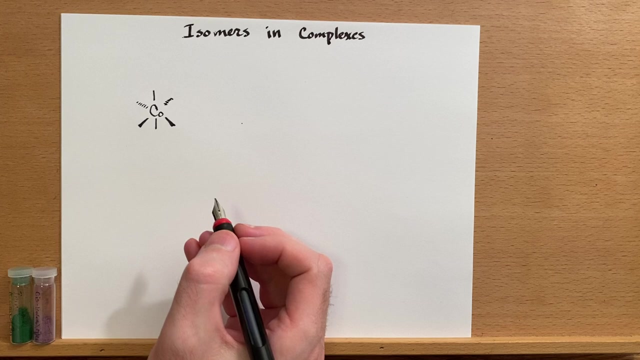 So we have cobalt, and then we have our octahedral geometry, and these are coming out of the page And these are really going into the page. I should have dashed that line too. And then these two positions are contained within the page. 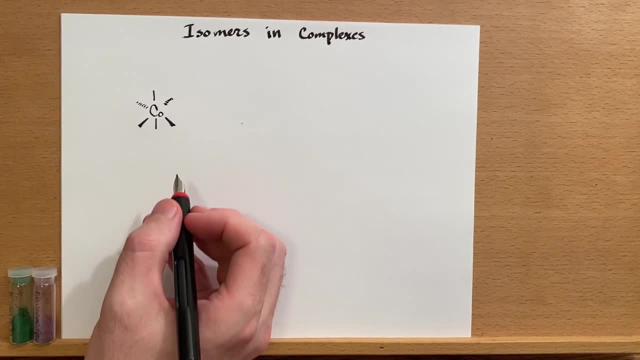 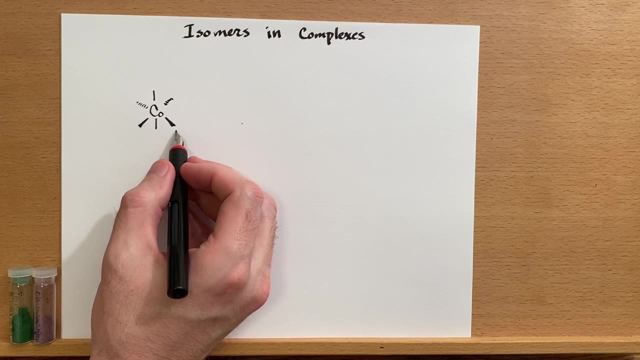 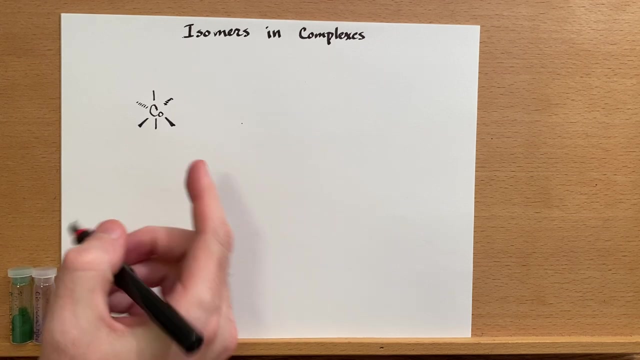 So cis means same side, And so these need to be on the same side of the metal. Now that could be these two positions, or those two or these two, just not on opposite sides. So if I put the chlorine here, I could not put it there, for example. 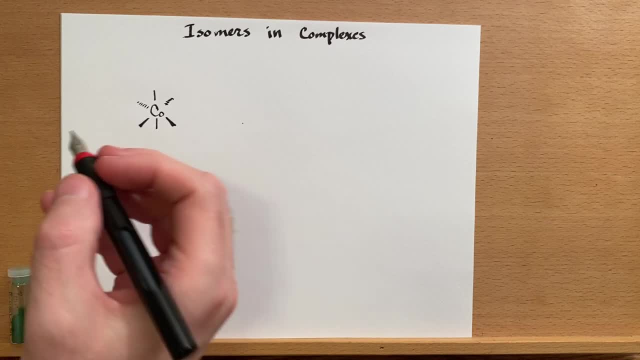 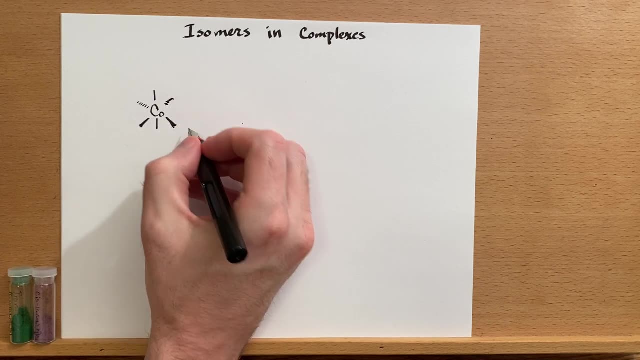 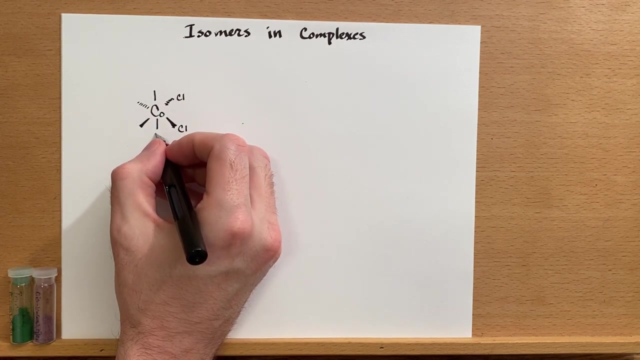 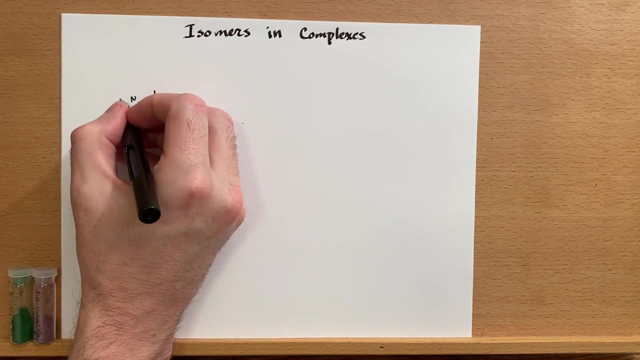 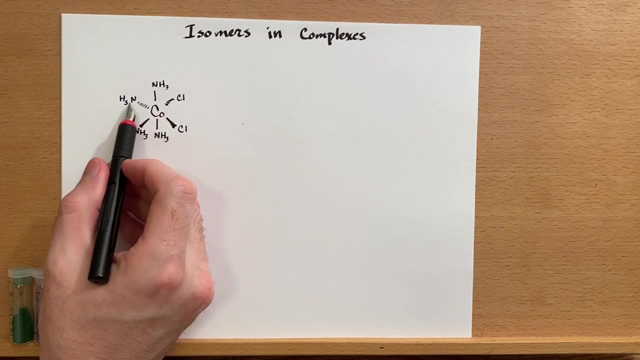 That would be the trans configuration. So let's just draw one of the options for drawing the cis configuration. So we'll put the Cls here and there and then the rest of the locations are going to have ammonias. Now you might wonder why I write this H3N. 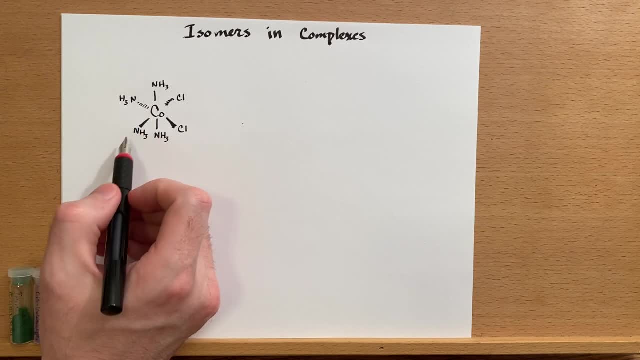 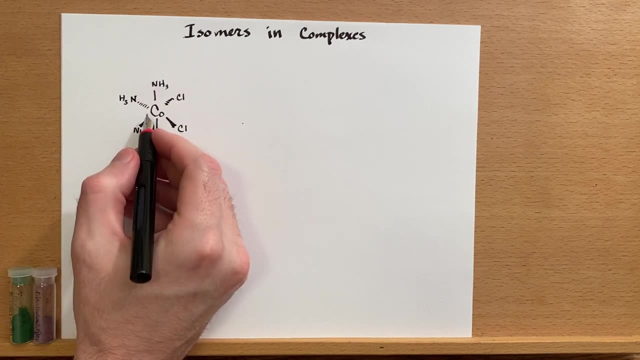 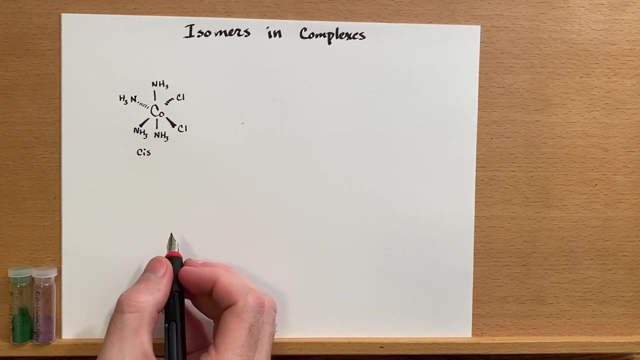 And that's simply because the nitrogen is doing the bonding to the cobalt And over on this side. it's just the way to write it. Now, this is the cis configuration, So in naming this we would just say cis tetraamine. 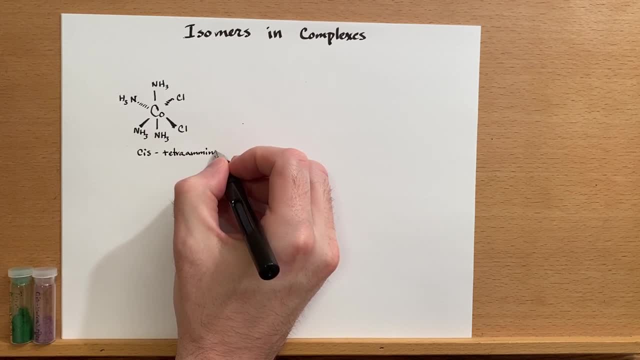 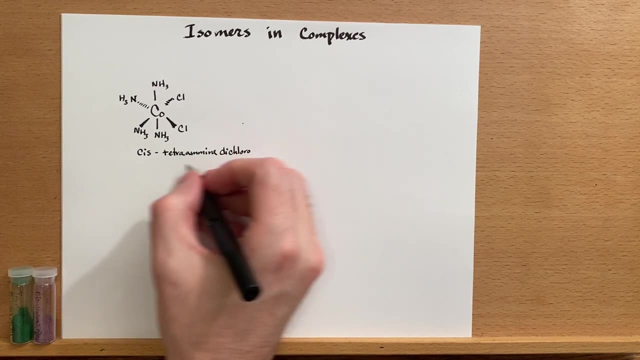 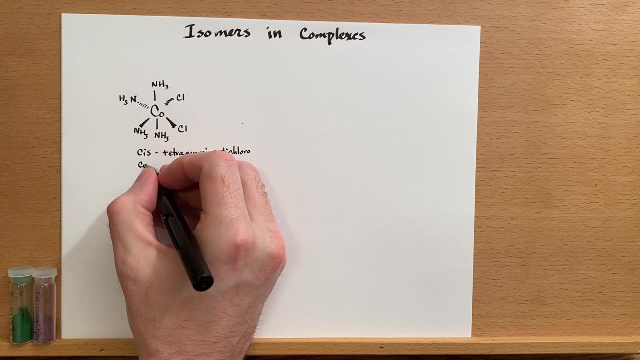 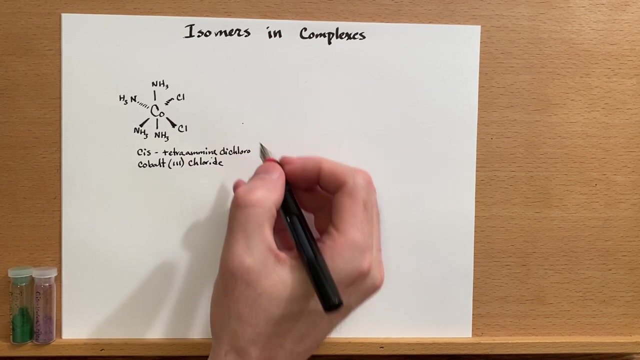 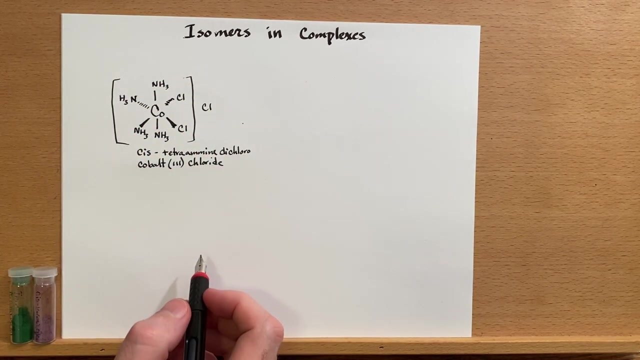 Dichloro Cobalt. I'm going to run out of space over here, so I'm just going to write it down here, Because this whole thing actually has. I'm going to put the chloride on the outside of it. So this is the cis configuration. 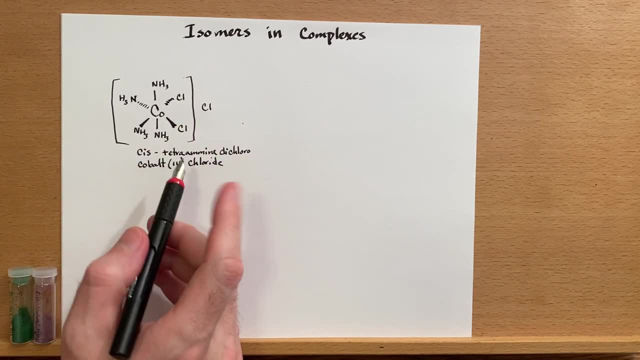 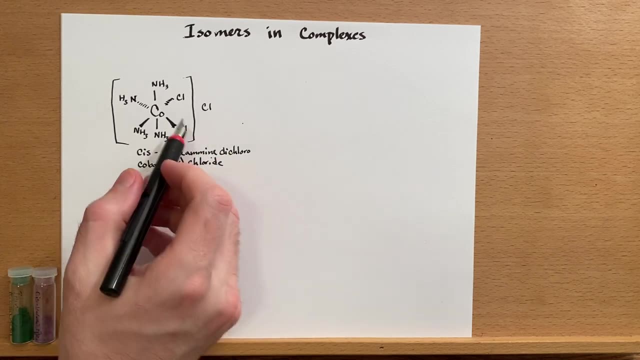 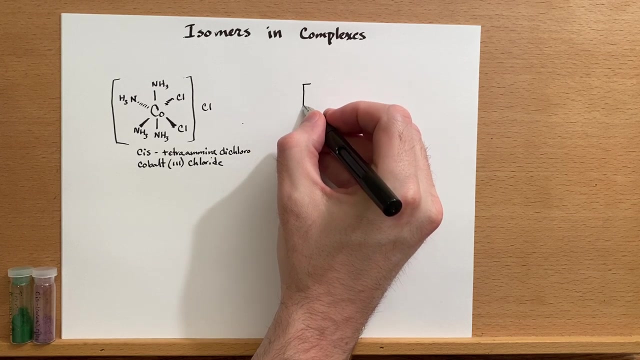 Same side of the structure And we could have actually put the chlorines here. We could have put them there Anywhere that they're not directly opposite. So let's draw the trans configuration And I think possibly in this case I'll avoid writing out the name again. 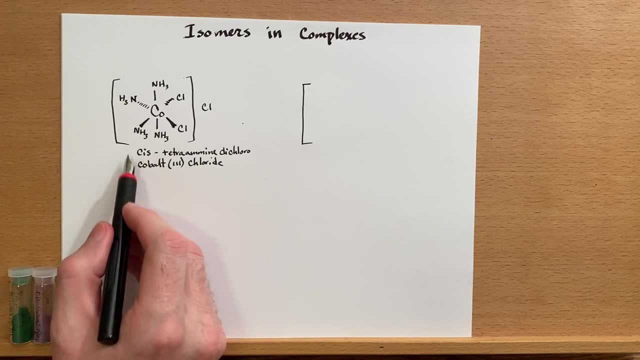 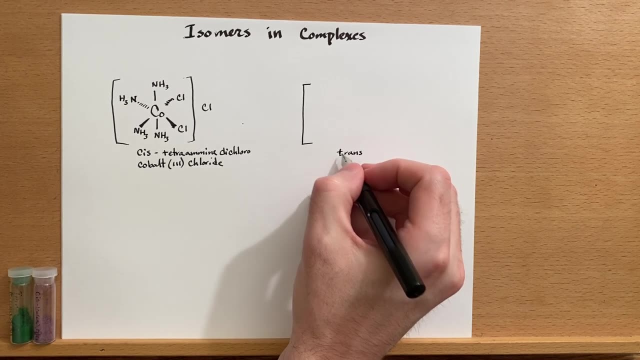 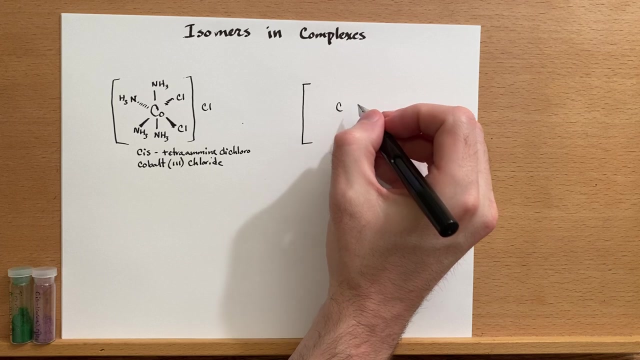 because the only thing that will change is just the cis will change to trans, So I'm just going to write the trans right here And then you'll know that it's still tetraamine dichloro, cobalt chloride. So we have cobalt. 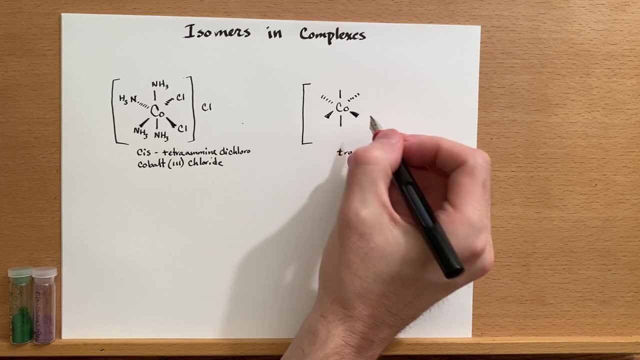 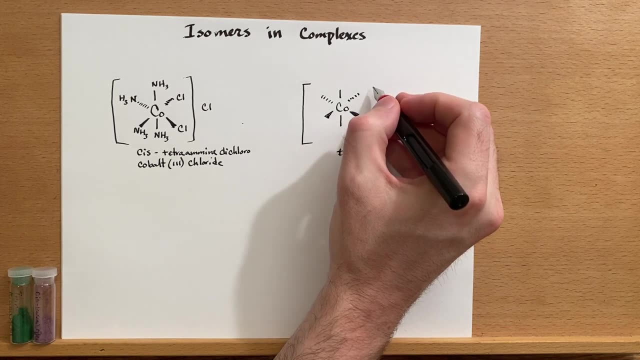 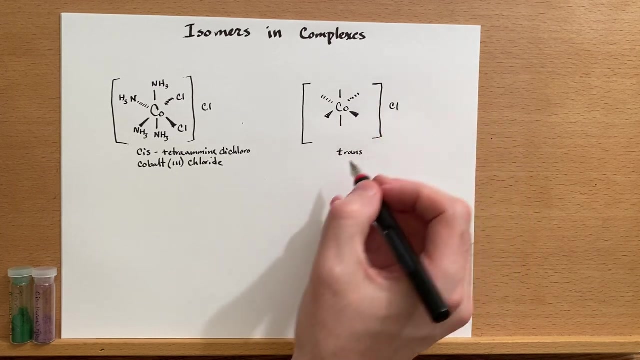 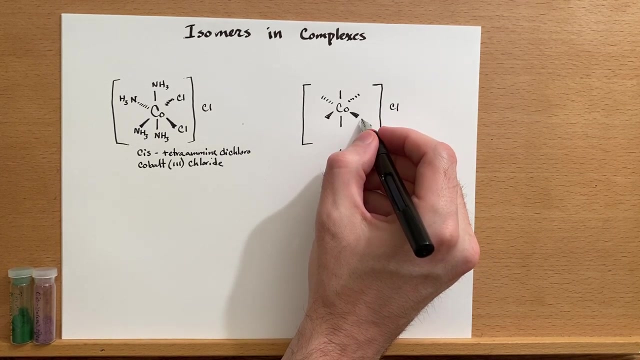 Just like this. Now, in this case we need to put the chlorines on opposite sides of the metal Still have a chloride out there. So it doesn't really matter where we put the first chloride, It just matters where we put the second one. 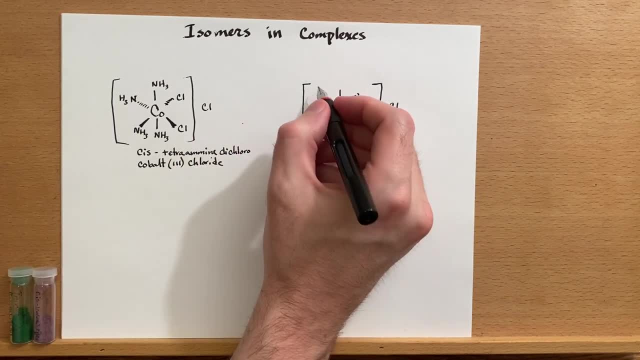 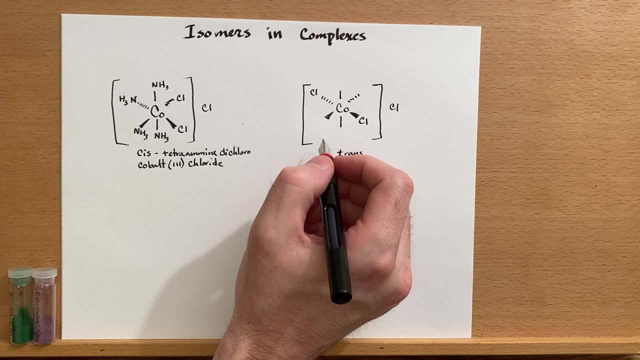 So if we put the first one here, say, just like we did over here, we'll have to put the second one right here, on the exact opposite side of the metal. If I put it in any other location, it would be the cis configuration. 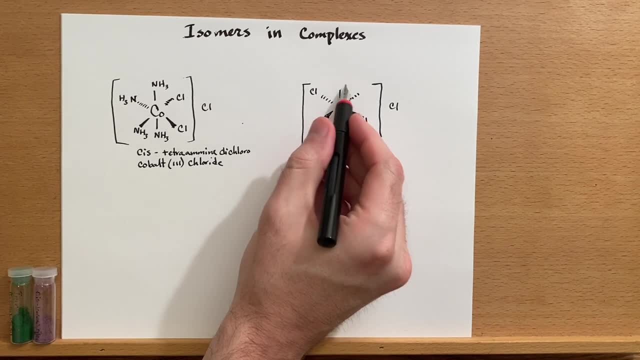 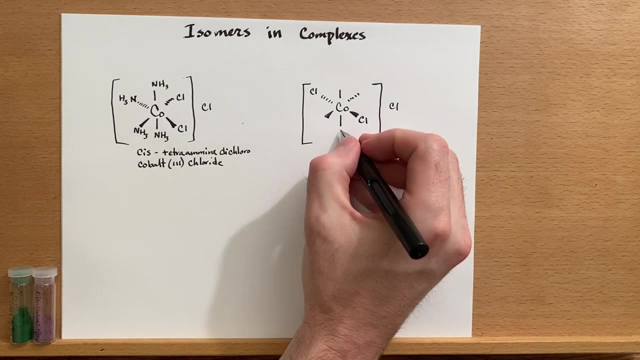 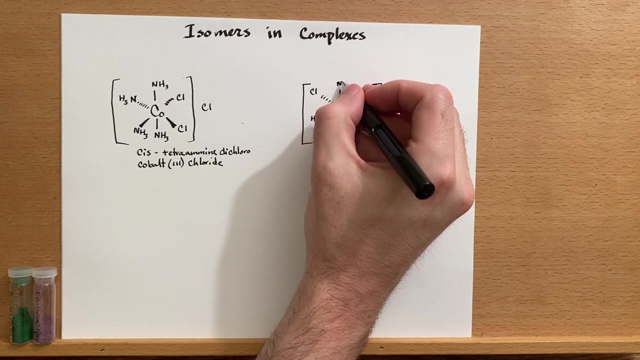 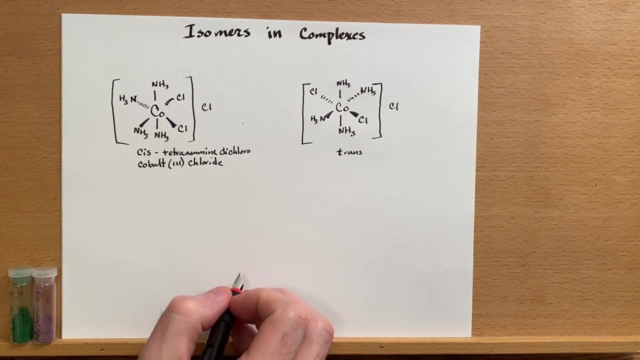 The cis drawing. Put it here, here, here or there. Those are all cis configurations, Only exactly opposite. is it the trans? And then we fill out the rest with our ammonias. Now, cis and trans isomers are not the only kind of isomers that we can have in an inorganic complex. 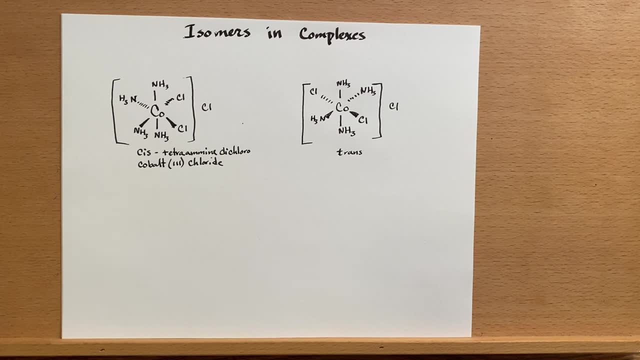 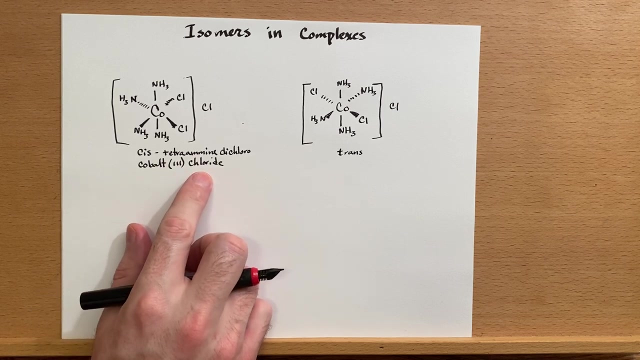 We can also have facial and meridian isomers. So what would that look like? Well, we'll have to change the complex. because tetraamine dichlorocobalt chloride cannot have facial and meridian isomers. We actually need three ligands that are the same. 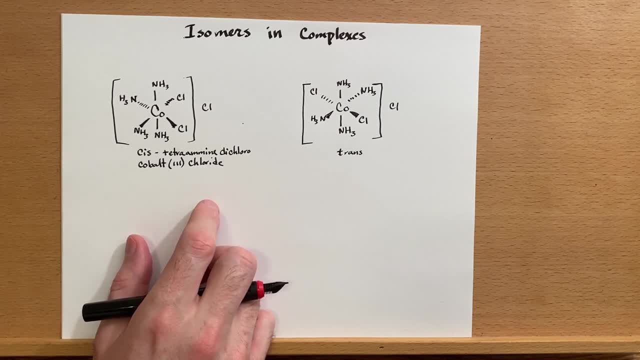 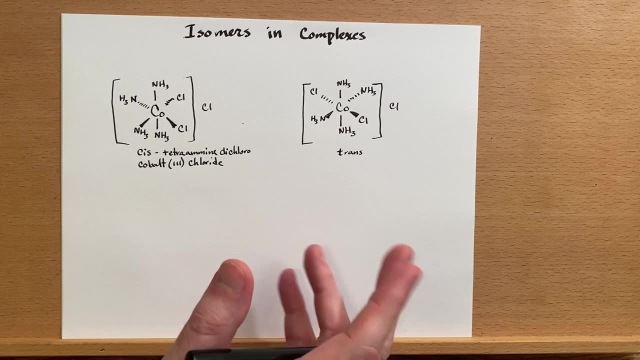 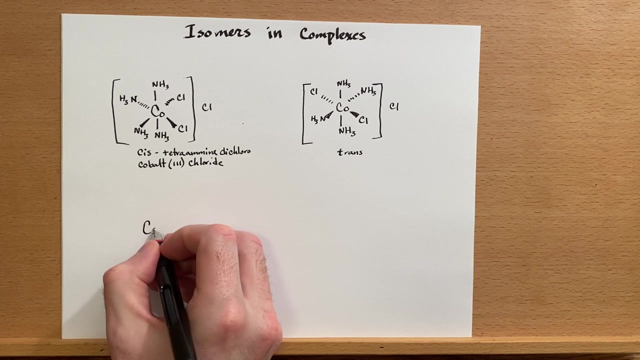 And I'll just keep the other three the same as well. So we'll have, say, triamine trichlorocobalt chloride And we'll draw that, And there are two isomers for this complex. So again, 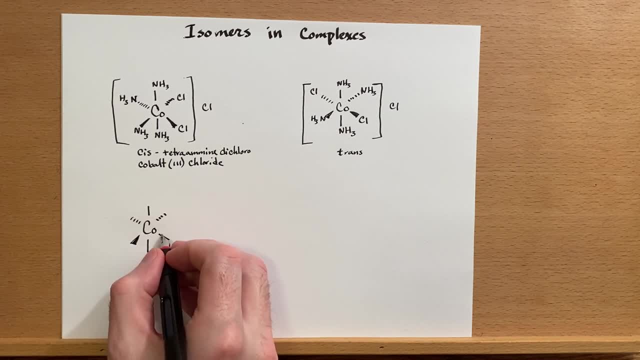 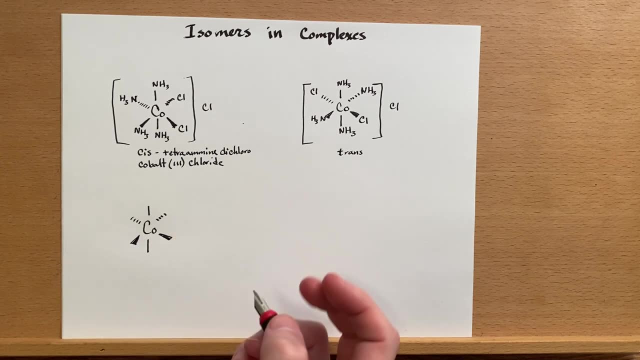 we'll draw our cobalt complex And in this case we have three chlorides and three amines to place around the complex. So let's draw the facial isomer first, because it's kind of similar to the cis isomer. 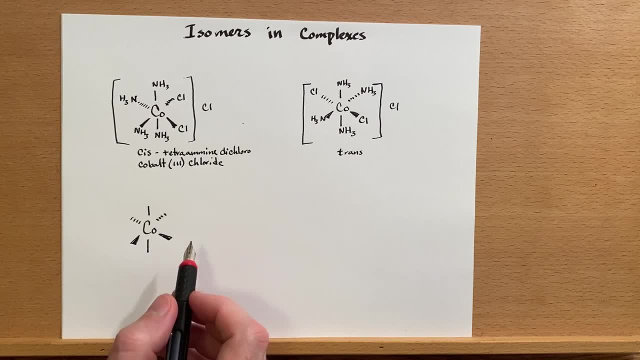 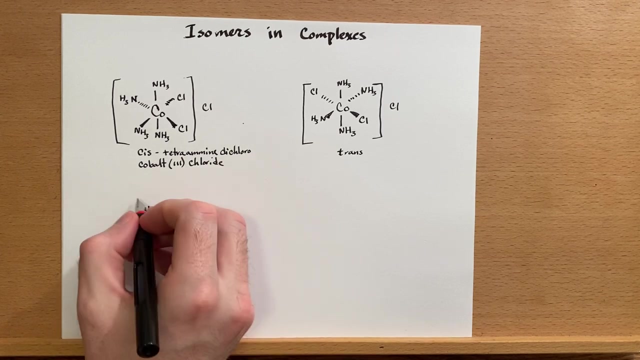 in that we have all of them on one face of the octahedron- I almost said tetrahedron- there, So chloride there, there and there, And these all form a triangle on one face. So this is the facial isomer. 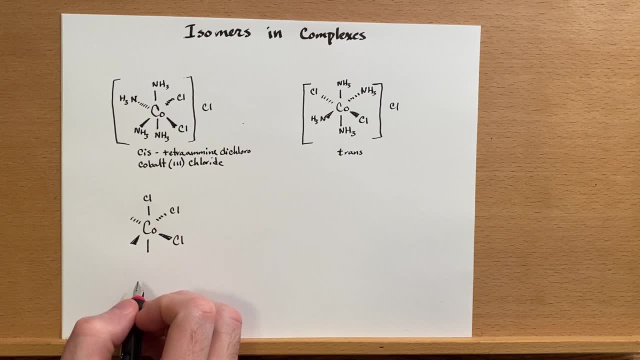 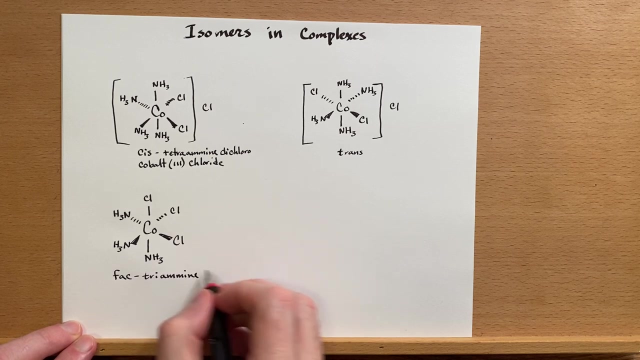 which is sometimes abbreviated FAC or FAC isomer. And then we have ammonias over here in the other positions. So to name this complex, we would have FACIAL ISOMER and then TRIAMINE TRICHLORO. 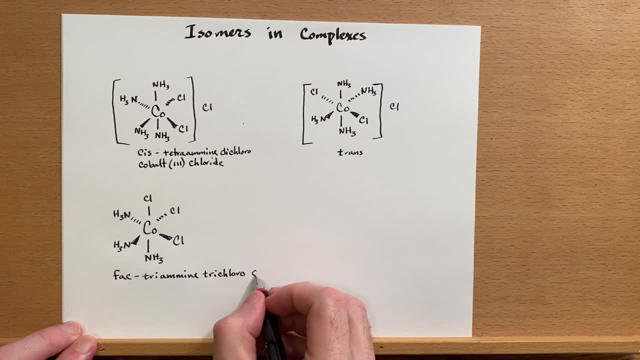 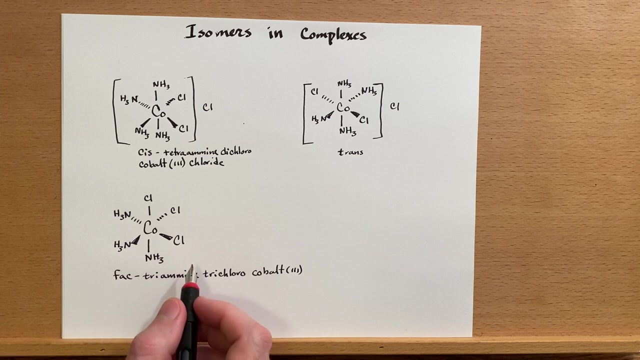 and then just COBALT 3. I think I can fit it. And since we have three negatively charged ligands- charged ligands- We don't have any other ligands in the outer sphere of this compound. So this is the facial isomer where all of one of the ligands are on. 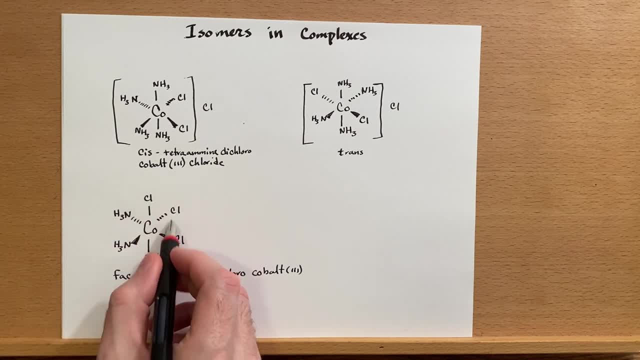 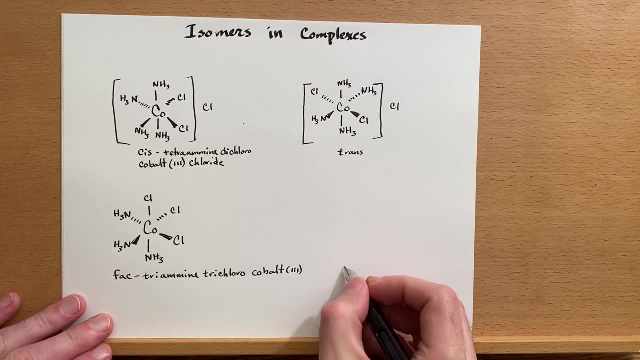 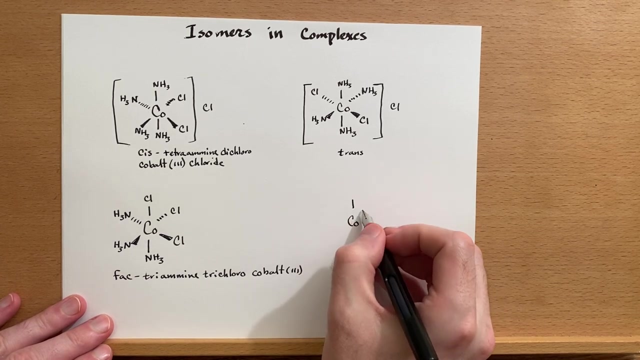 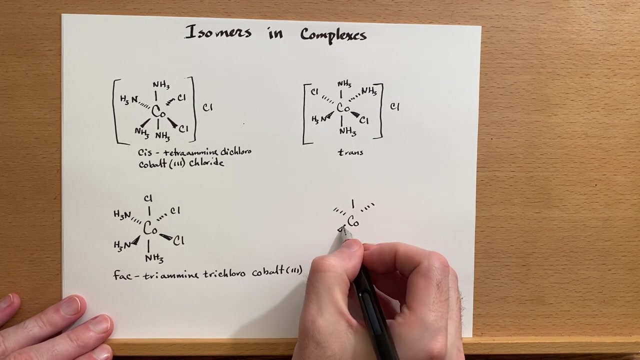 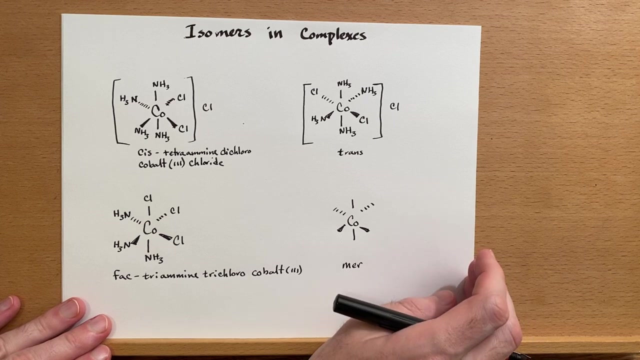 one face. We can kind of draw a triangle here. that's one face. And then we have the meridian isomer, which is abbreviated into M-E-R. So let's draw that one and see if we can see the difference. Okay, So for the meridian isomer, we can keep the chloride here. 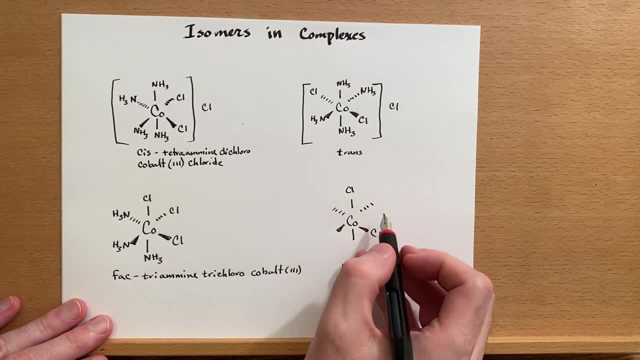 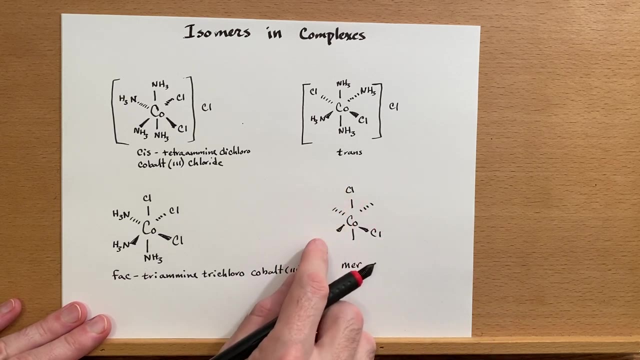 And then we have ourisanė clove. we can keep one here, but we can't put it there because that would be the facial isomer, just like we had here, right, and we can't put it there because that's just a face, like that's the facet facing us. we could put the other chloride. 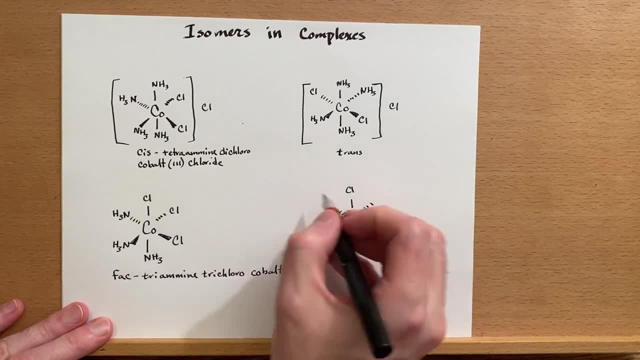 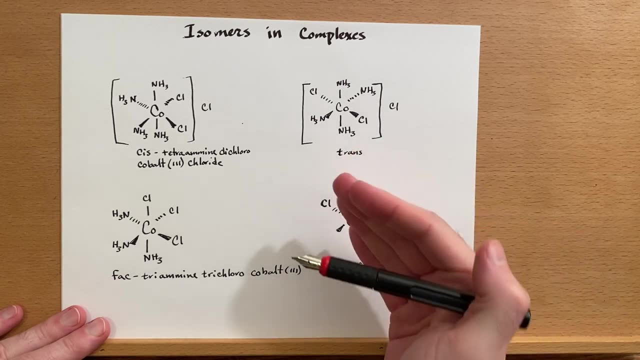 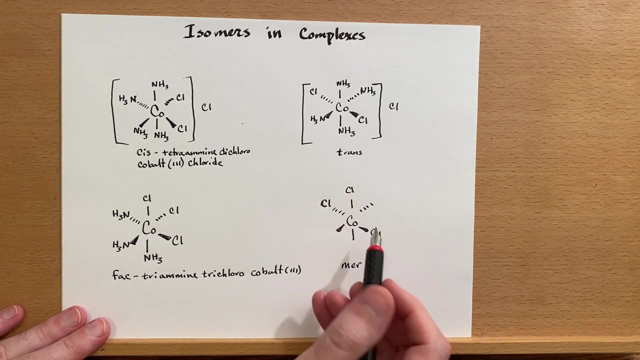 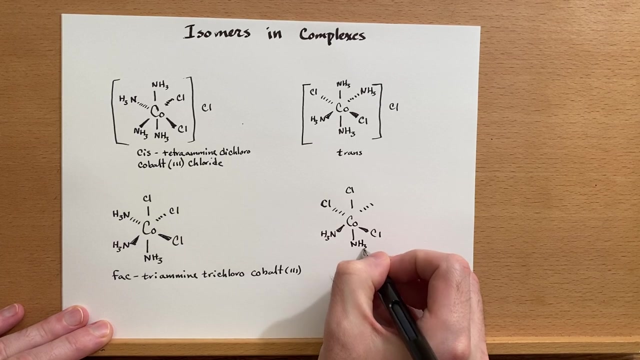 either here or there, so I'm gonna actually just stick it right here and now. these are all in one meridian, or the way I've drawn it. these are all in this plane, one, one straight line in each other, and and then we would put the ammonias in the other position, and these are all in one line. 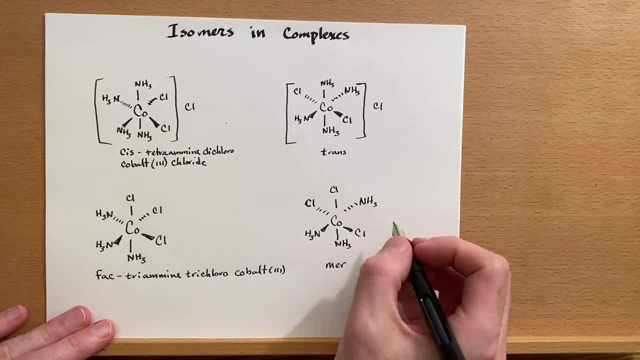 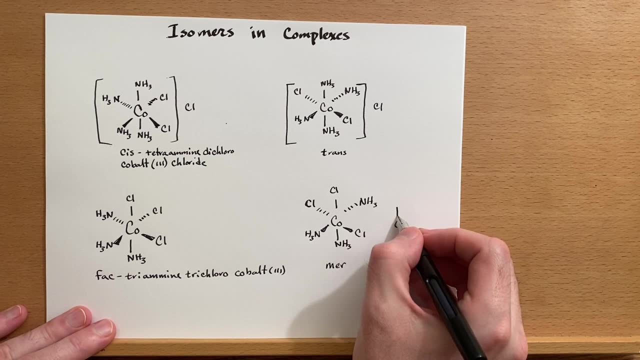 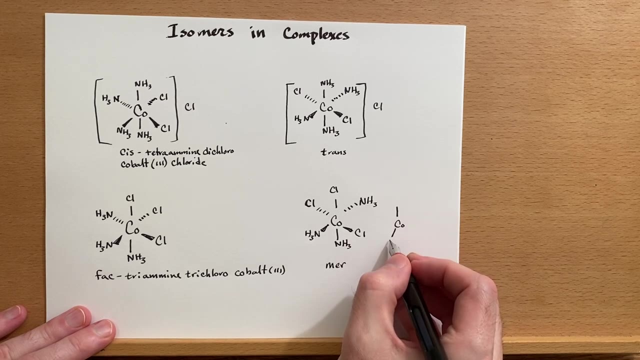 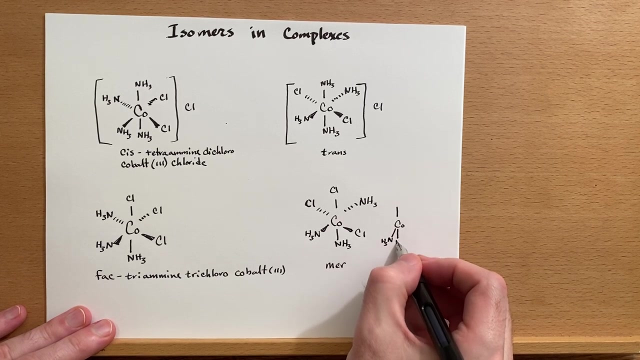 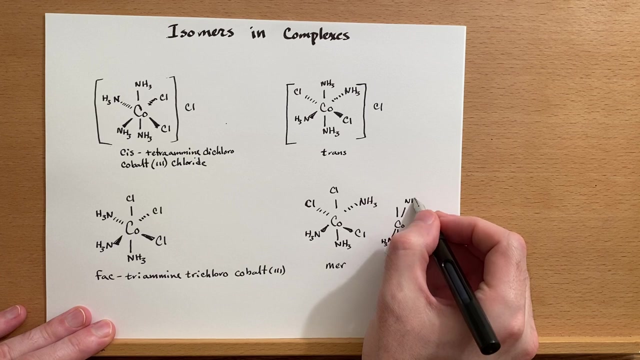 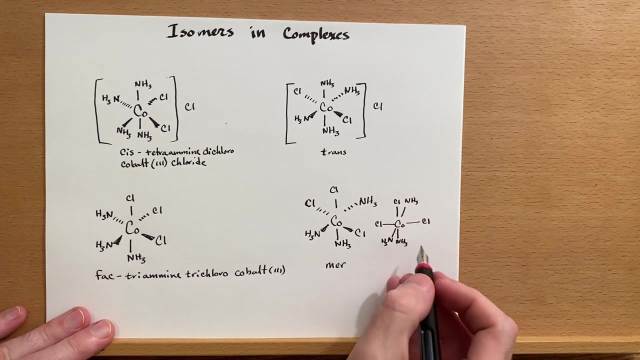 you. so let's draw. let me draw another view of this, maybe a little bit more edge on. so let's see, here I'm gonna draw this very skewed and then that's, that's gonna be like way back there, and then my CLs are like this. so in this case I've drawn the CLs as the plane of the paper. 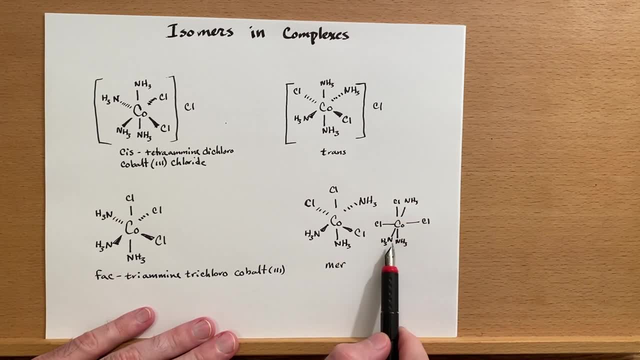 and then the ammonias are all like this one's coming out of the page and that one's going in and out of the page, and then the ammonias are all like this one's coming out of the page, into the page right. so these are all in one flat meridian right, one plane. 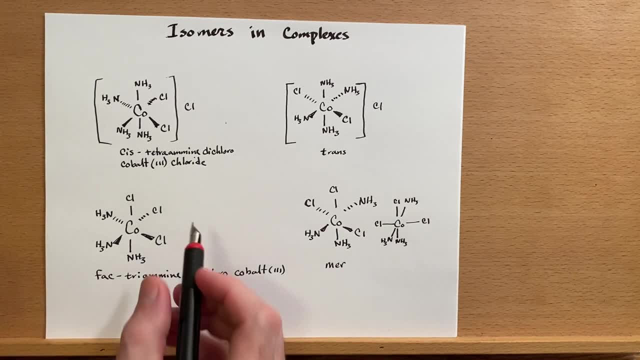 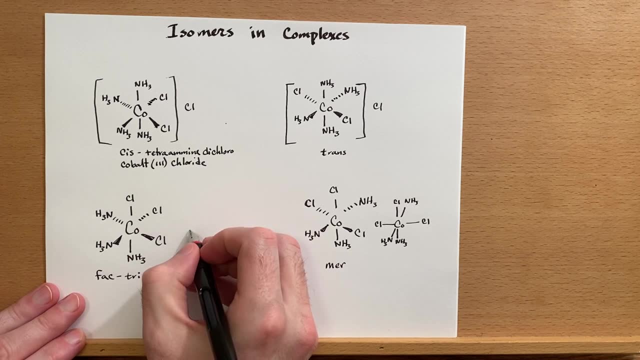 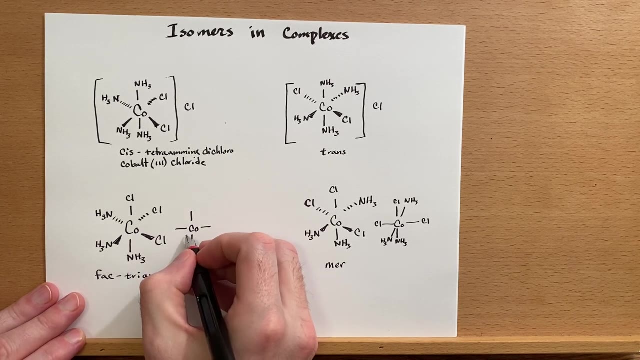 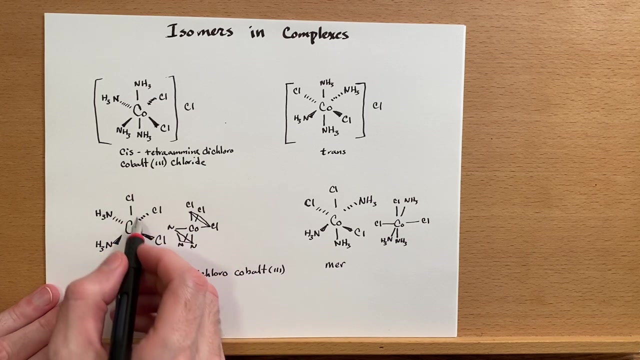 and these are all contained in the same plane. now, if I drew the same thing over here, it would look like this. so these are all on one face, so there's like this triangle here. actually, I could probably draw the triangle a little better over, at least over there, but this is all on one face of the octahedron. maybe it's better to just muddy up this picture right over here by drawing the triangle like this. 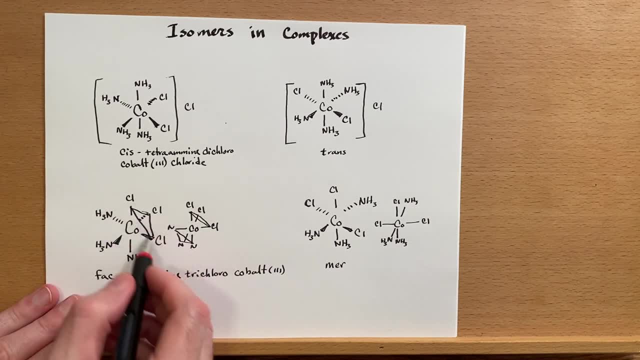 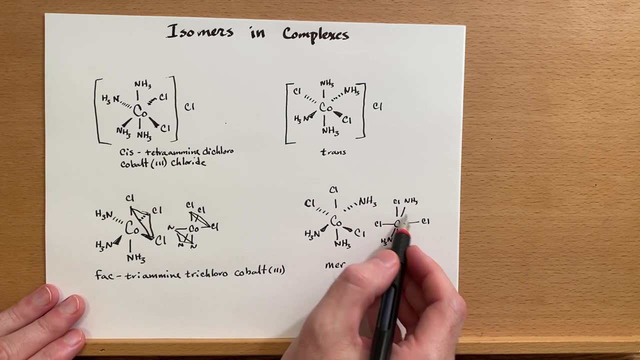 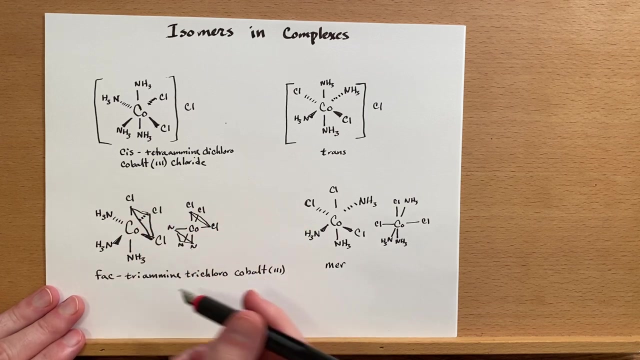 right, see how there's. there's all in the same triangle. I can't do that over here, right? if I try to draw the triangle on this one face, I will have one of the nitrogens or one of the ammonias contained in that triangle. same thing, like I can't draw like one straight line and have it all be chlorines over here. chlorine, chlorine, ammonia. 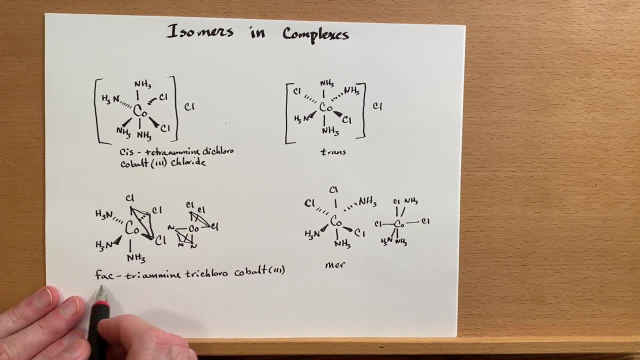 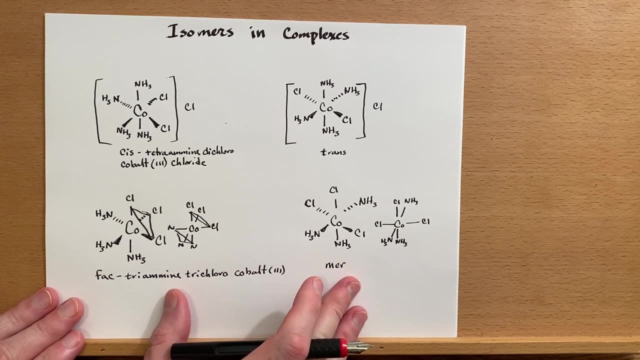 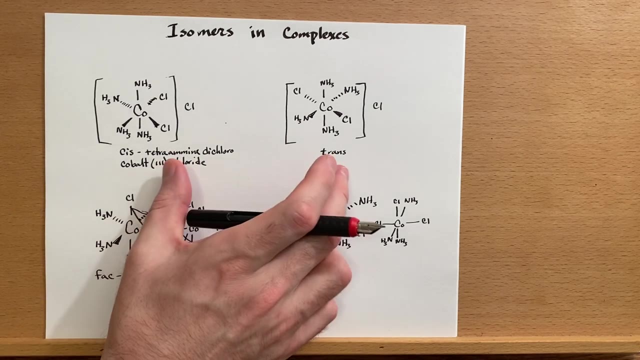 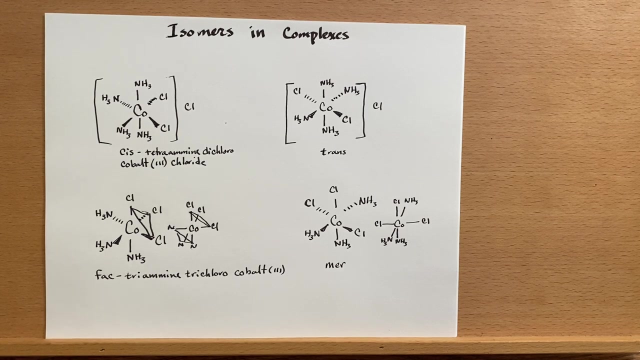 so this is a different isomer. this is the facial isomer, that's the meridian isomer. these particular isomers are possible in an octahedral geometry. now cis and trans isomers are also possible when we have a carbon with another double bond. so there's no rotation about the carbon bond. but 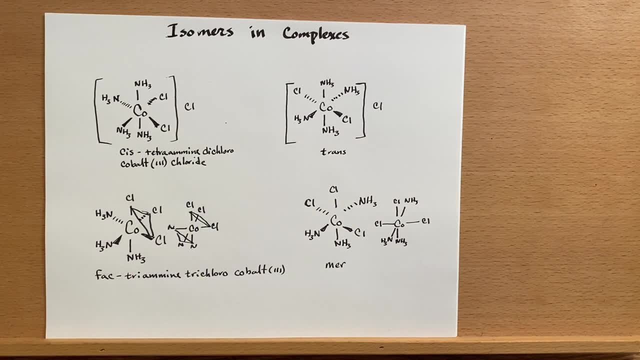 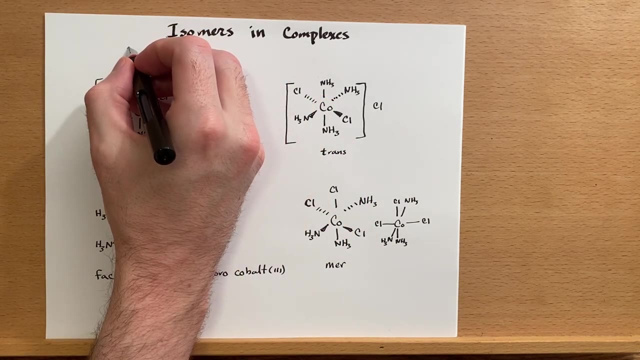 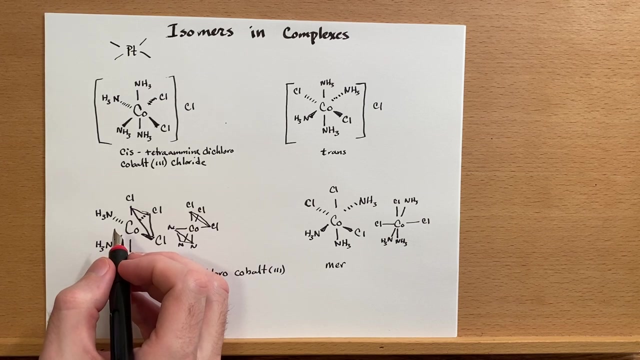 you can also have cis and trans isomers in inorganic complexes. this is possible. cis and trans are also possible when we have square planar complexes, such as when we have a platinum complex. now, this is square planar, so it's just one plane and you can have. 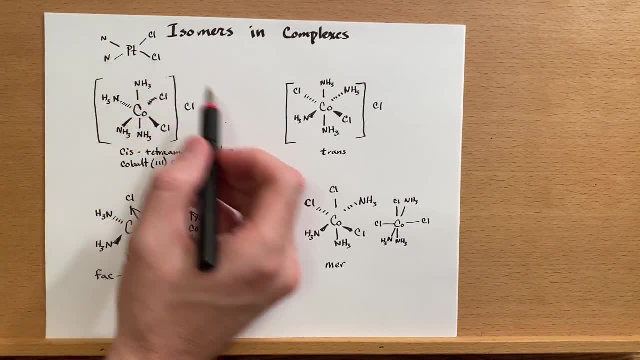 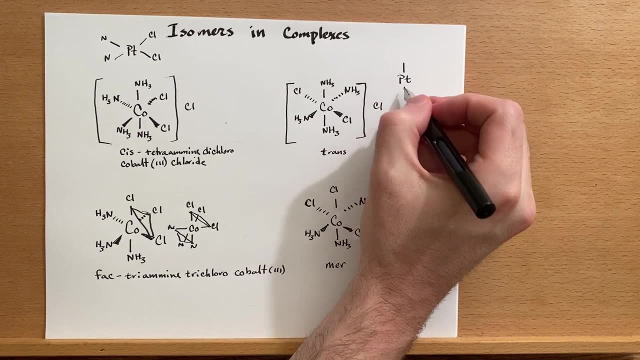 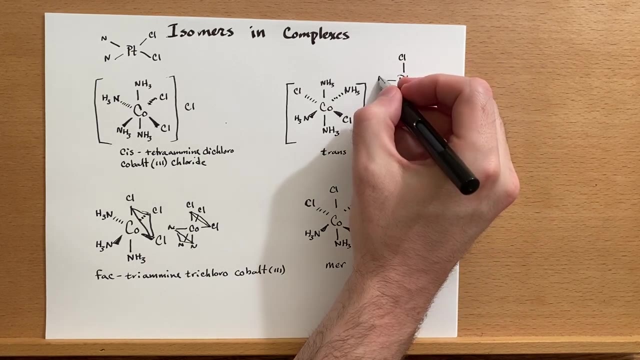 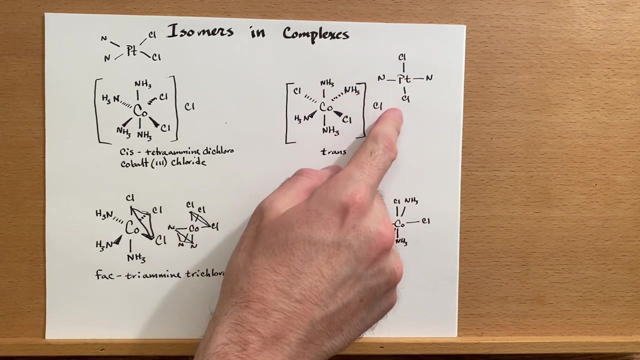 a complex that looks like this, where they're on the same side, and you can also have the platinum with the, with the trans. I'm just going to draw this one kind of looking down at the top of the molecule and I'm leaving off all the hydrogens, but you get the idea they're on opposite sides of the molecule and this would be trans. 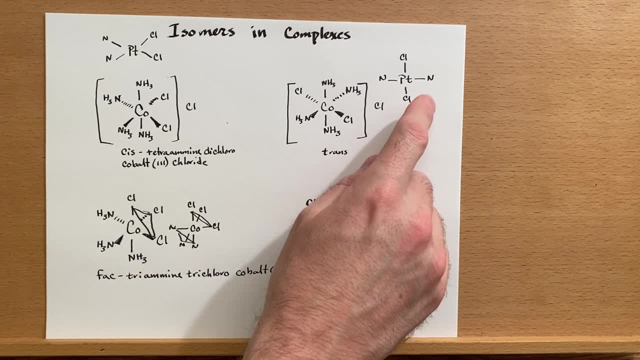 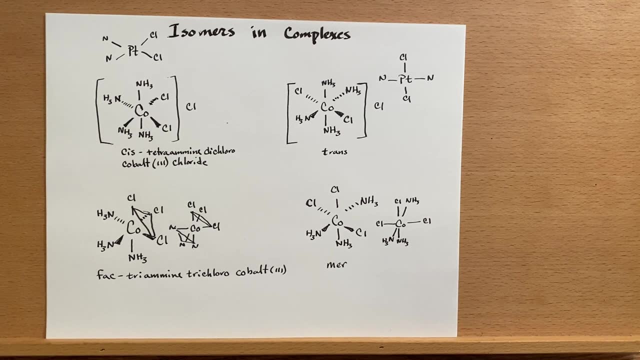 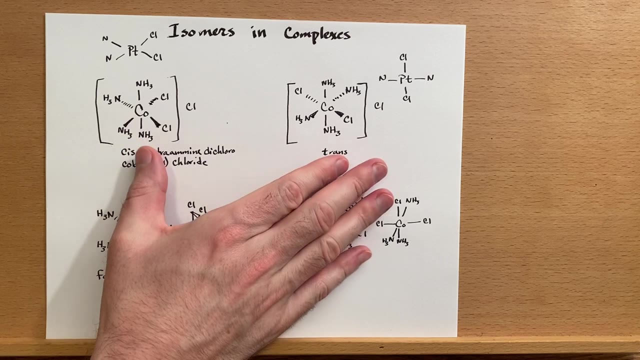 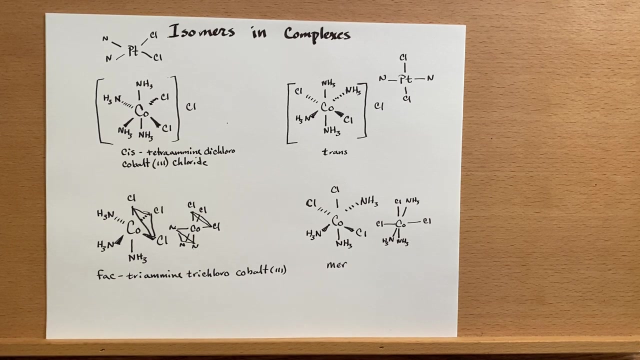 cis configuration, trans configuration in square planar. tetrahedral geometry does not have a cis or trans configuration, but octahedral and square planar do. and then octahedral further has the facial and meridian isomers. now it is also possible for us to have